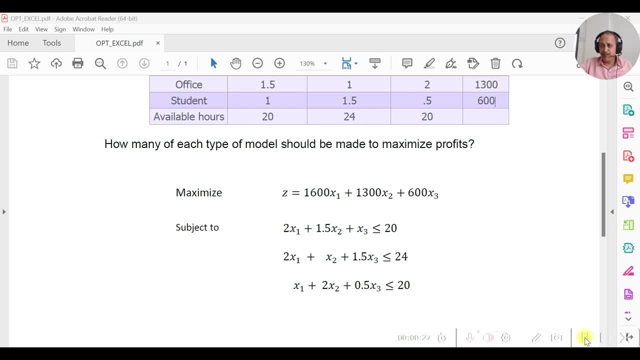 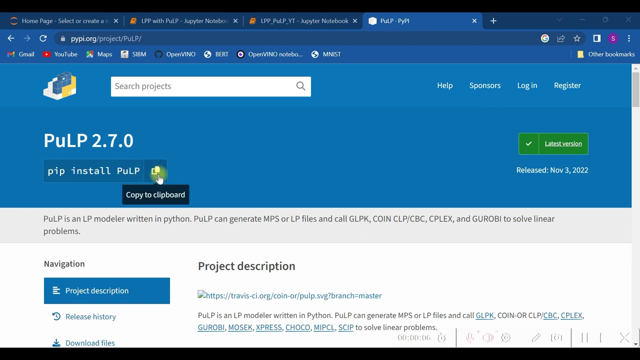 formulated. This same problem was also taken as an example in one of our earlier videos with Excel option. Let us do the same thing now with Python pulp package. Now, to begin with, please ensure that you have installed the package pulp in your Python environment. 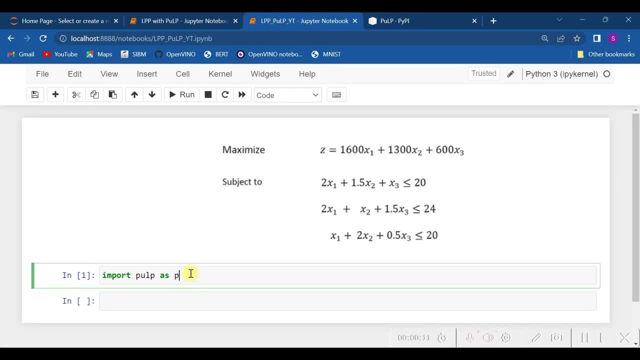 Having installed pulp in your Python environment, you need to import pulp With import pulp and alias you can give. preferred alias can be p. As this problem is of maximization, you need to first of all specify that particular thing with the option lp- maximize. Let us do that, Hence we have written over here. 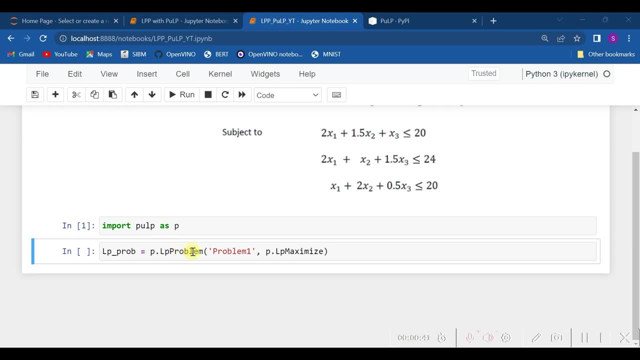 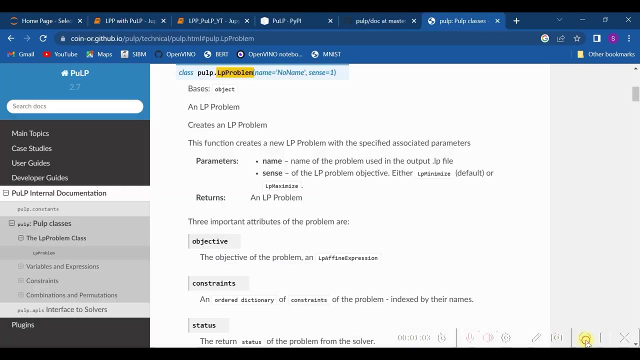 called over here the function p- lp problem, in which we can give any name. The string is optional. Actually we can give any name to it, as I have given over here as problem one. But if the problem is of maximization, please do not forget to specify lp or p- lp- maximize. We are using version of pulp over. 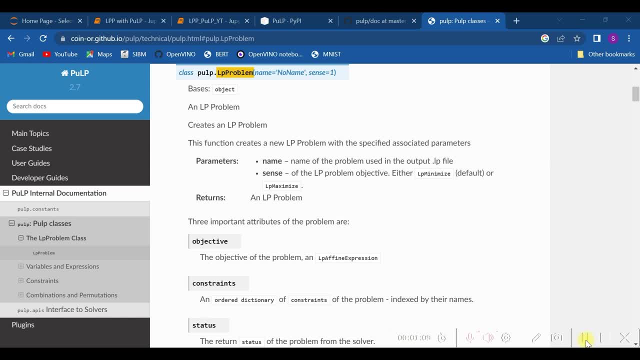 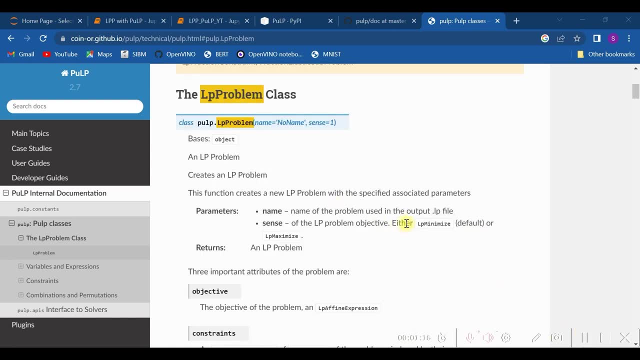 here as 2.7.. And you can very well see the documentation. Also, you can see one thing: that if you do not specify whether you need to minimize or maximize, the default option is: lp, minimize Now. having executed this, we now required to define the. 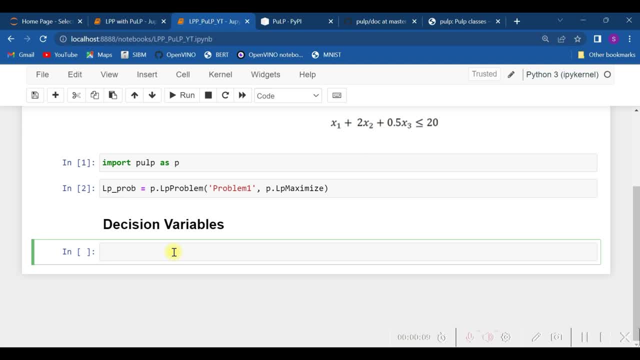 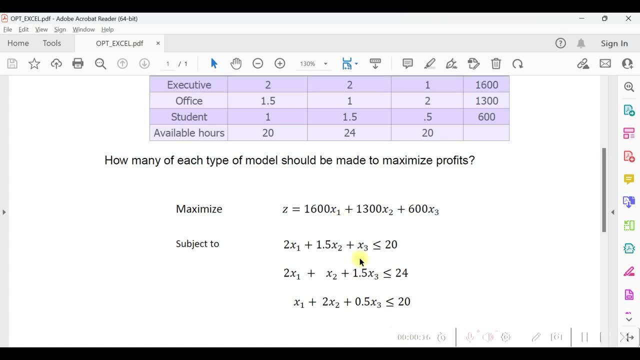 or specify the decision variables. As you see, in our problem the decision variables are three decision variables: x1, x2 and x3. now, while we specify it, mind it well that over here we have product mix problem. so none of the variables should be over here less than 0. 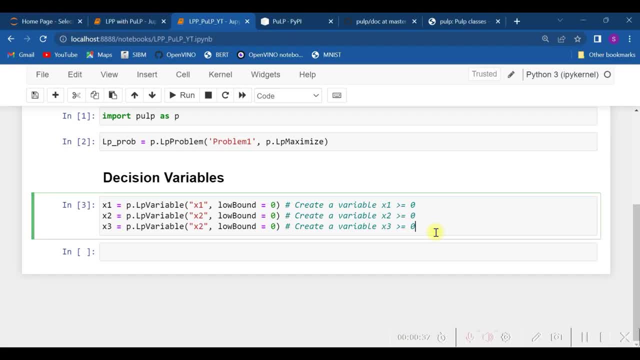 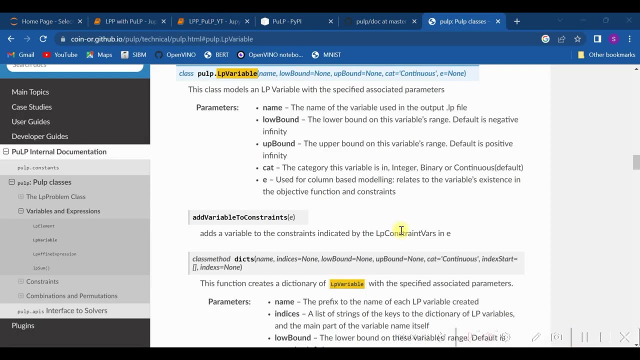 it can be 0 or more than 0 and hence the bounds have been given. as you see, we are calling the variable, we are calling the function lp variable for defining the variable. if you check documentation of that particular function, you will see that there is a provision of giving upper bound as well as lower bound. so in case, if you require, 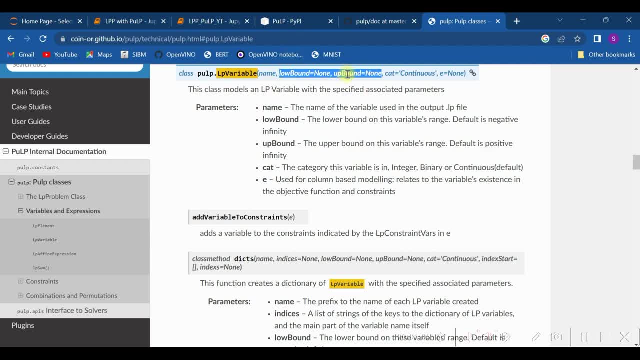 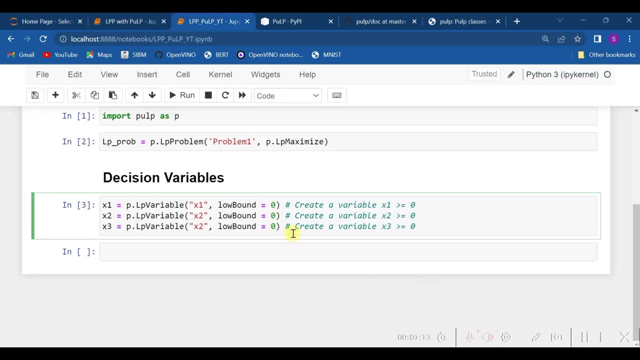 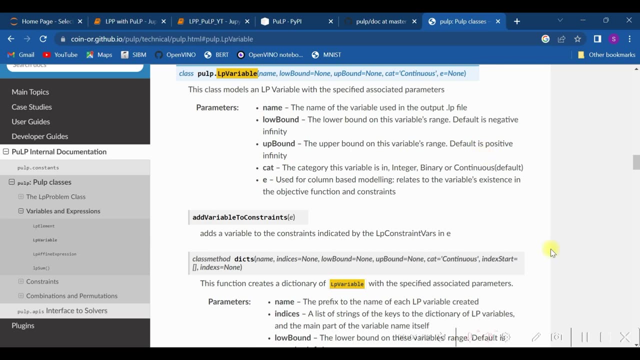 to give upper bound, then you need to specify it with the option up bound. so if you require to give upper bound, then you need to specify it with the option up bound. here we have specified low bound is equal to 0 and no upper bound option. that means up bound can be positive infinity. there is no bound for up bound over here. 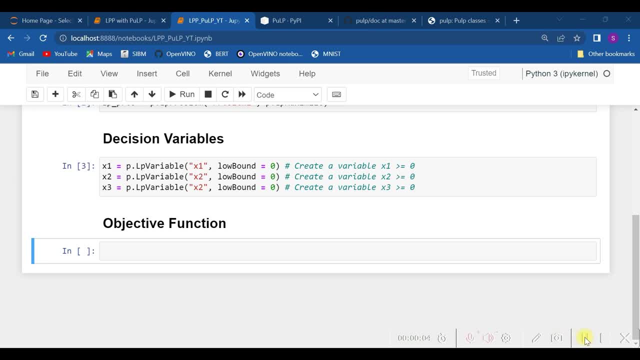 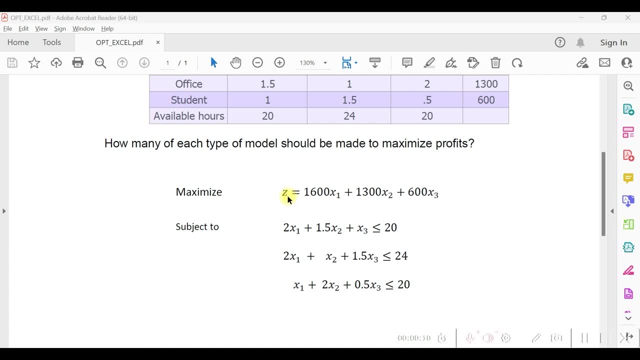 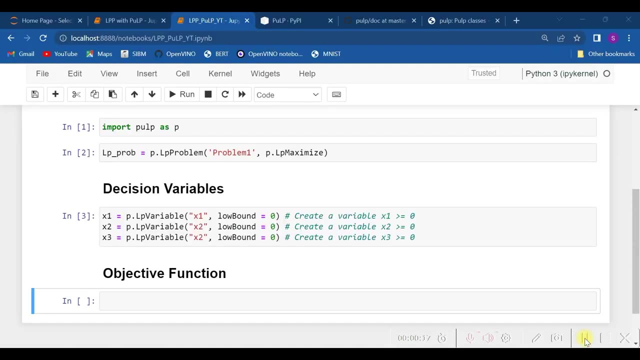 having considered defining decision variables, let us see the objective function. as you see we have. the objective function at z is equal to 1600, x1 plus 13 and x2 and x3. over here let me tell you that entire problem of our lpp is going to get stored in the object. 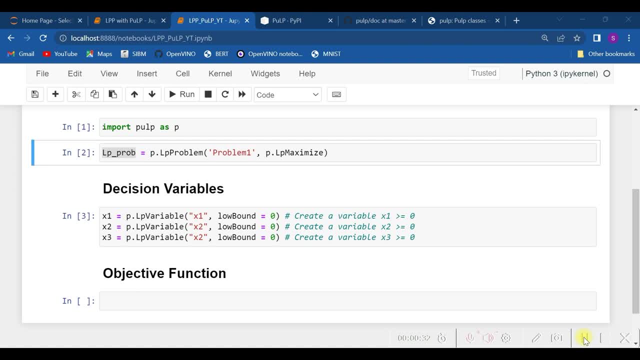 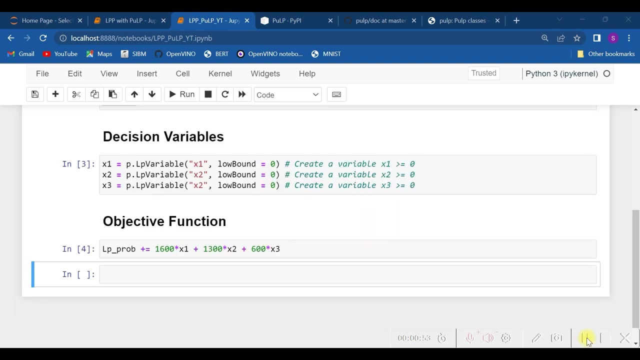 lp prob. lp prob. we have already defined here as the maximization problem in lp prob. lp underscore prob object. we are going to now specify the objective function with the syntax plus equal to: let's do that. hence, as you see, the objective function has been specified with lp underscore prob object. next come the constraints. 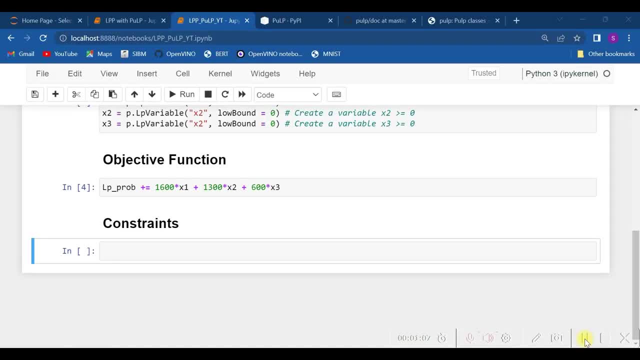 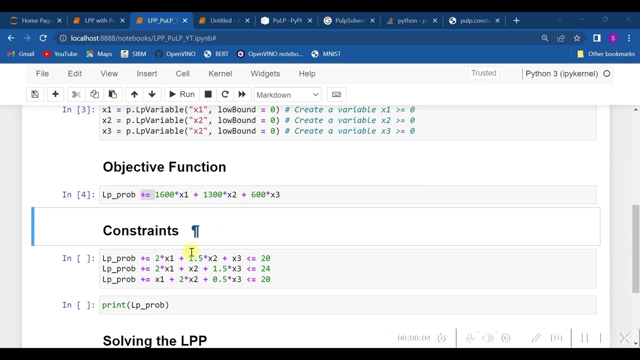 every constraint needs to be specified with inequalities or equalities. if equalities are there, and, as i had said, all the constraints also need to be specified with lp underscore prob object, let's do that. hence, as you see, the constraints have been specified and once the constraints have, 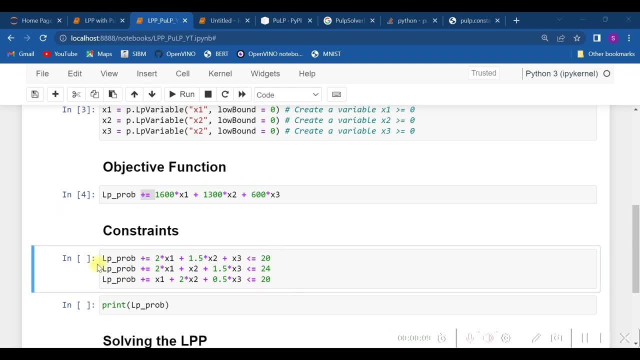 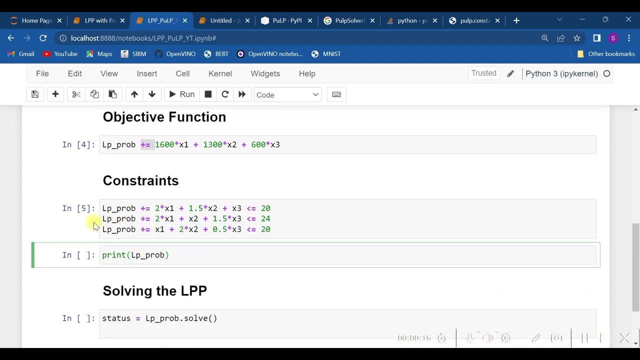 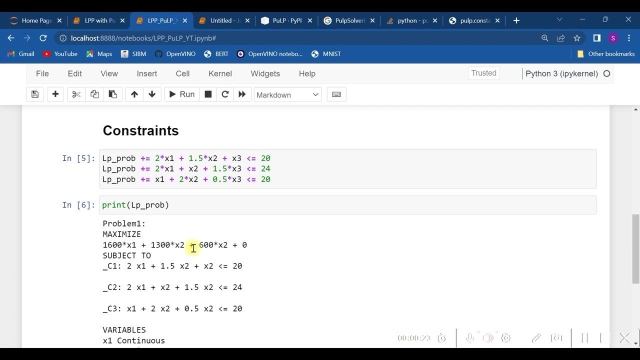 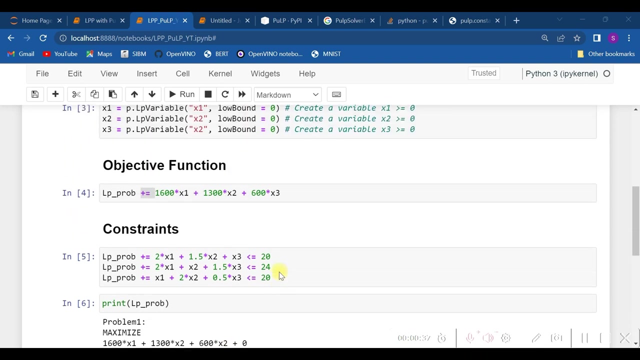 been specified over here. we also need to check first of all whether we have entered everything properly with lp underscore prob problem. you see over here one problem, one typo which might be there, is that we have specified x1, x2 and x2 and not x3. we need to check it by scrolling up and here comes our bug, so we need to correct it. 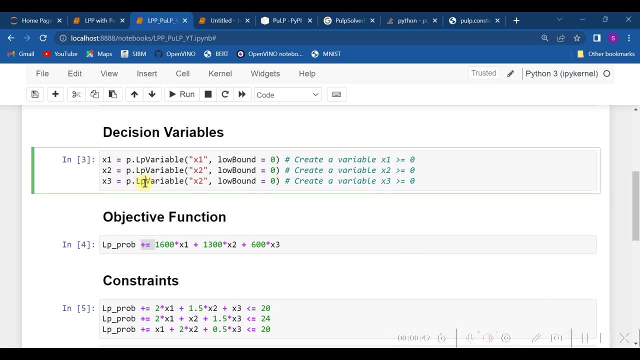 so, as you see, it's not just enough to name this x3, the. it's necessary to have x3 over here because the LP variable, the LP variable or I can say also LP prop, recognizes the object name specified over here. hence let's edit it and again run it. before we edit and run, please make sure that the 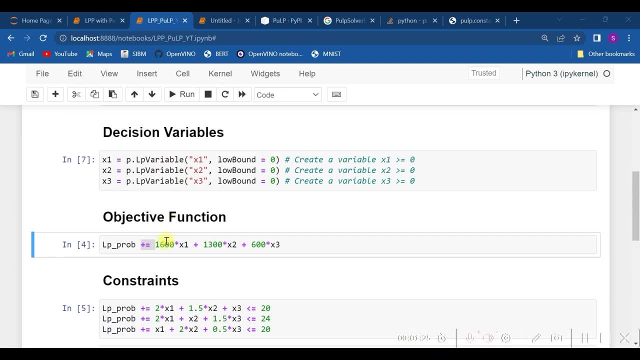 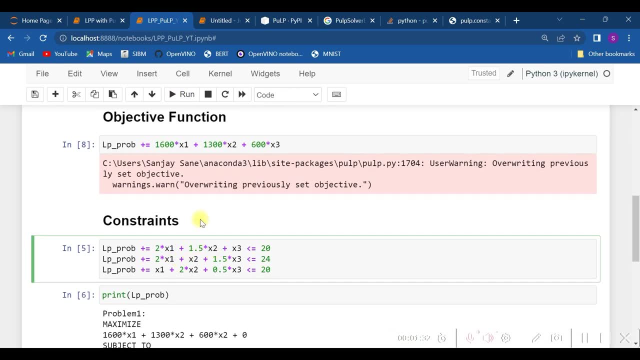 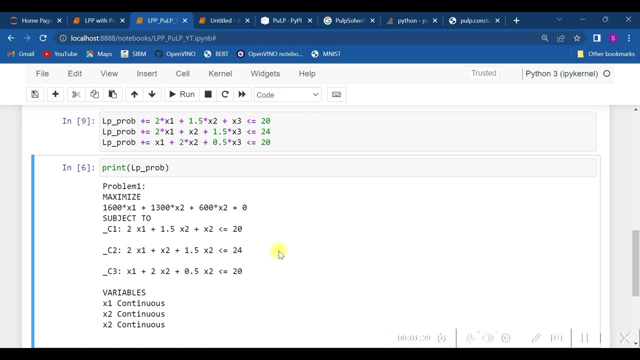 variables which you are entering are not getting entered twice, for example. now one more problem has occurred: we have overwritten certain things, ok, and hence some few more variables have been added. so still the things haven't been corrected. so my suggestion is: when you make any change over here, 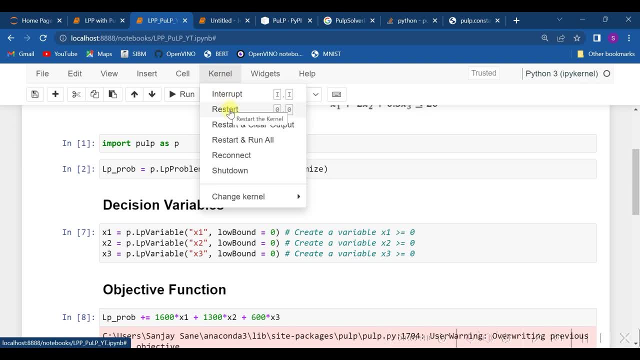 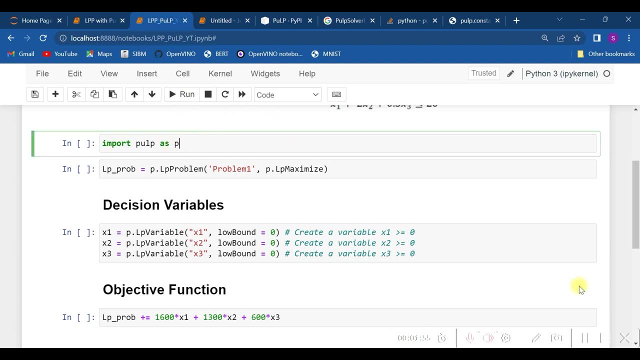 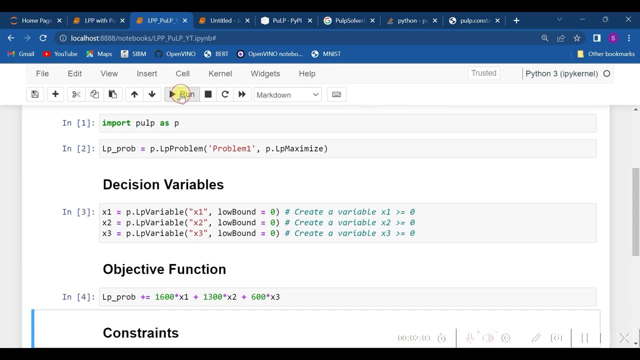 up here, better it will be that you restart and clear output and restart and run all that will be more better choice. so hence, having done this, having done this correction, i am going to run this run, this run, this run the constraints and again check whether i have entered everything. 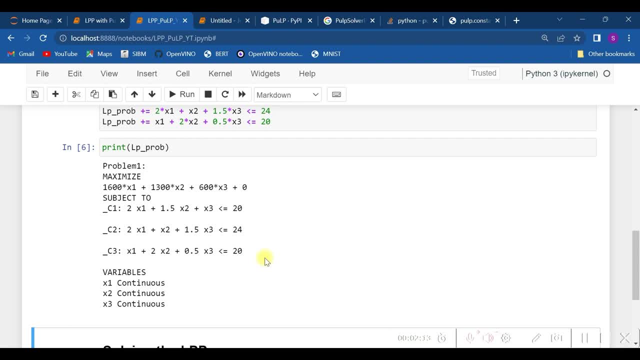 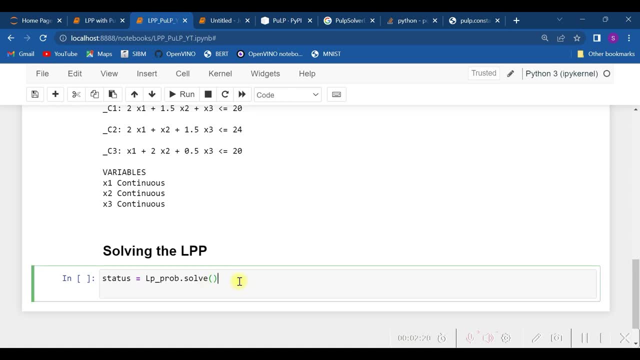 properly or not seems. this is okay and fine. and now we are going to solve the problem. for solving the lp underscore prob, we require to call lp underscore prob dot solve now when we are going to solve. not necessary that every time our problem will result in optimal solution. it may happen that, you know, our problem will end in. 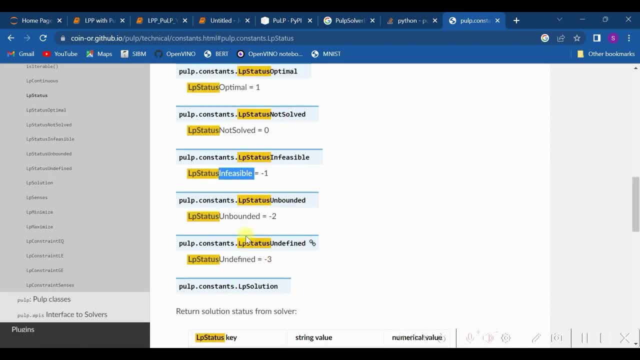 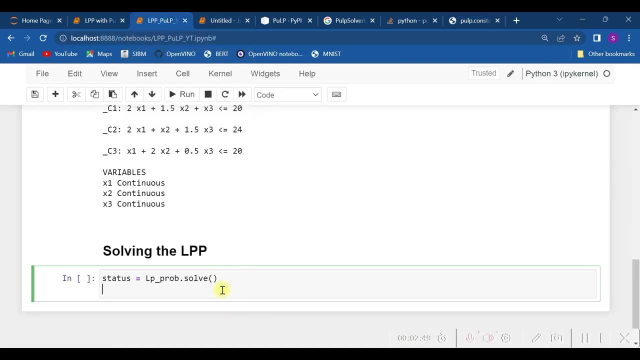 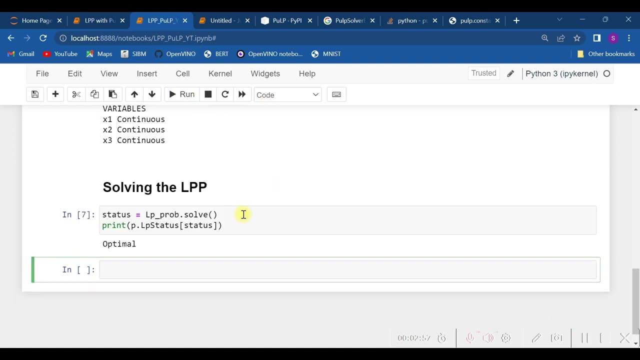 some, some non-solved, not solved, infeasible, unbounded, or something like that. we need to check that. how to check it out? with lp status function. so hence, as you see that our problem is having optimal solution, let's see the solution. let's retrieve the solution now for getting the solution. 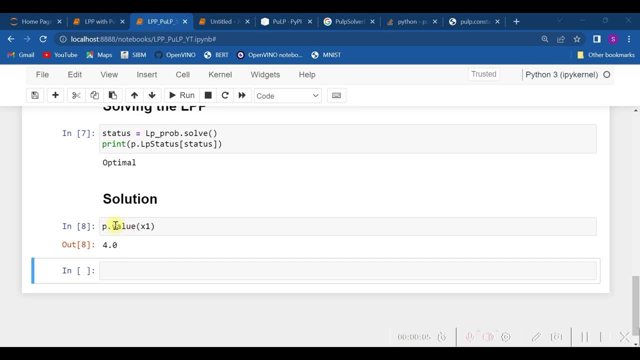 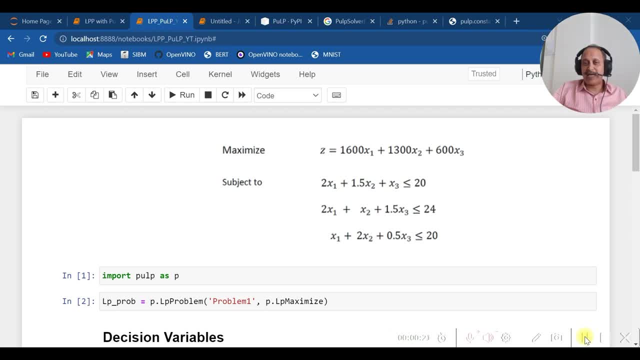